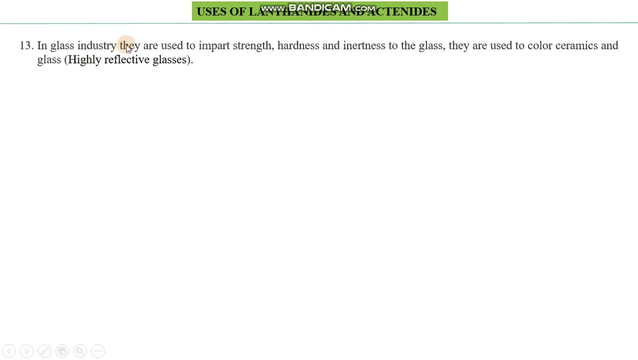 The next use is in glass industry. They are used to impart certain properties or attractive properties to glass. So, for example, strength of glass can be achieved by the use of lanthanides and actinides. Hardness in a particular type of glasses can be achieved with the help of. 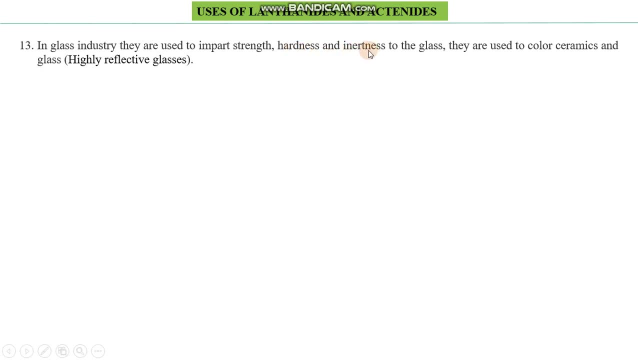 lanthanides and actinides. Their inertness, where they are used not to react with species, are in an environment which is rich in chemical species where the reaction between glass and those species is possible. So in that case the use of inert glasses is mandatory, and 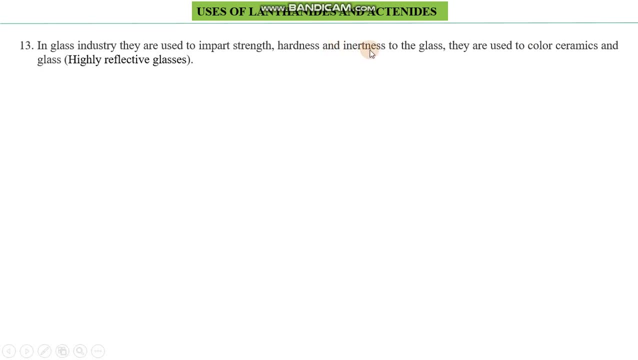 lanthanides and actinides are used to design such inert glasses. Now they can also be used during the color of ceramics. So this is again an industrial process. Some special method or special procedure has to be adopted in order to use lanthanides. 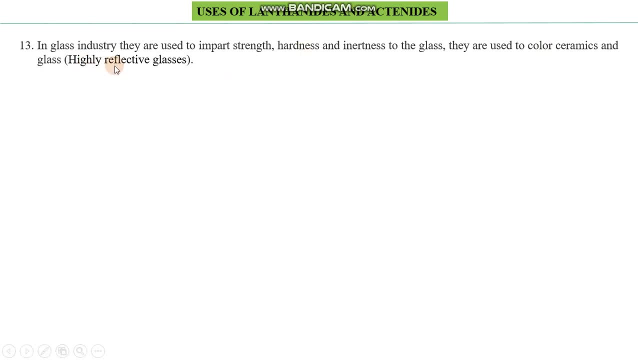 and actinides, And high reflective glasses can also be obtained by the use of lanthanides and actinides. So in electronic industry it also has some certain applications, For example production of red colored TV screens. So for example production of red colored panel technology over the light이�text II. 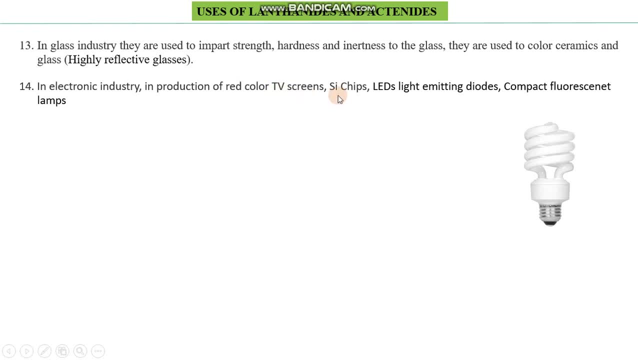 screens products, ie conventions in the electronic industry or, more specifically, solar observation systems From the view of superior space. you know how to become more intelligent And in disputable future, you can start to develop relations between around. possible because of use of lanthanides and actinides. silicone chips are possible because 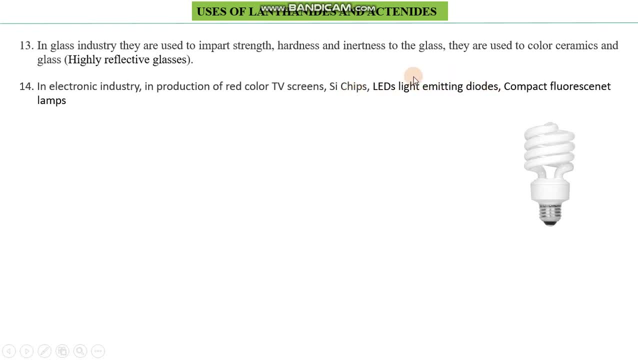 of lanthanides and actinides light emitting diodes. they are used in the production of leds and compact fluorescent light. so this is incandescent light and we are usually and normally using it. our homes, our offices, are other institutions such type of lights. so this is 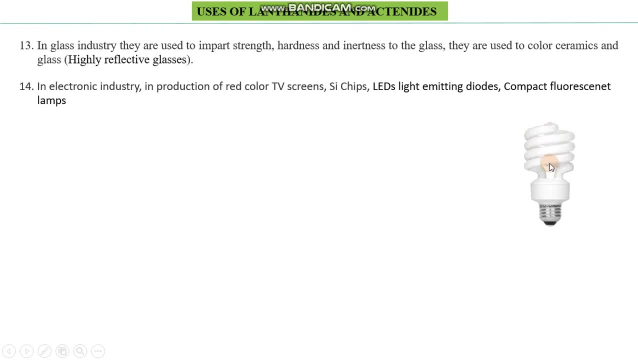 incandescent light light, and lanthanides and actinides are used in the production of these lights. these metals are used in the production of uv resistant resistance glasses and optical lenses. so this is again a useful use of lanthanides and actinides and the most useful use of lanthanides. 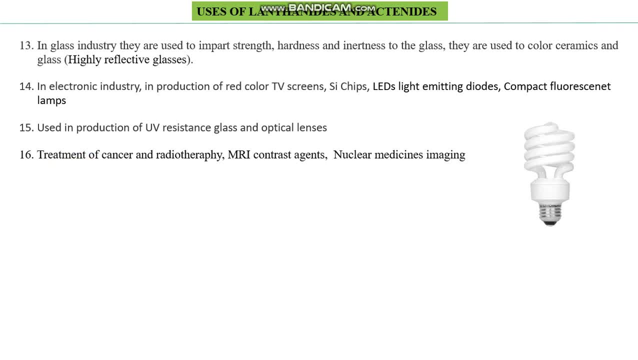 and actinides in the field of medicine so they can be used as in radiotherapy of treatment against cancer. radiotherapy is- this is a technique where where cancer is treated, this can also be used as mri contrast agent and in nuclear medicine it is used as imaging reagents. are imaging nuclear medicines. 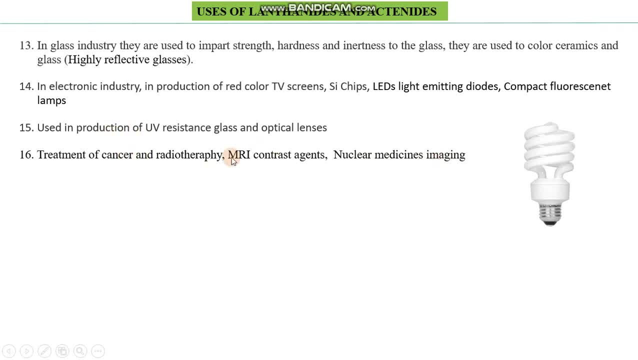 are produced or formed due to the use of lanthanides and actinides, because now, if you look so, radiotherapy is possible because of the use of those species which are radioactive, mri contrast agents. again, they are those species which are radioactive and nuclear medicines. so the name indicates that indefinitely. they are those species. 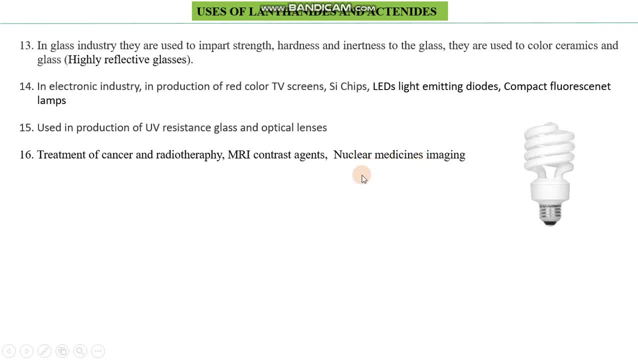 the medicine contains certain radioactive materials so they can be used because the lanthanides and actinides- most of them- are radioactive, particularly actinides. they are used to alter some electronic properties of compounds, for example electrophilicity. if we want to change the electrophilicity of 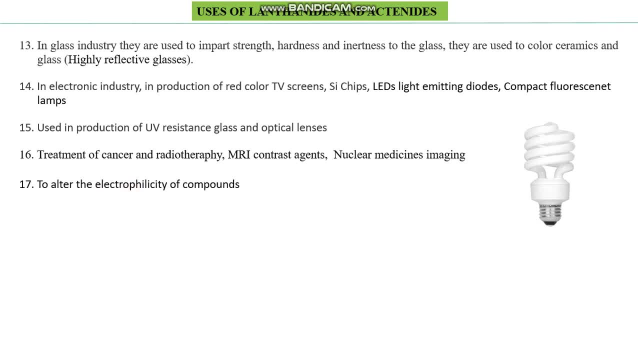 compounds in a desired manner. then we have to use lanthanides and actinides in automobile industries automobile exhaust system. they can be used for the purpose of catalytic converter. this catalytic converter is used to minimize the emission of carbon monoxide and carbon dioxide to 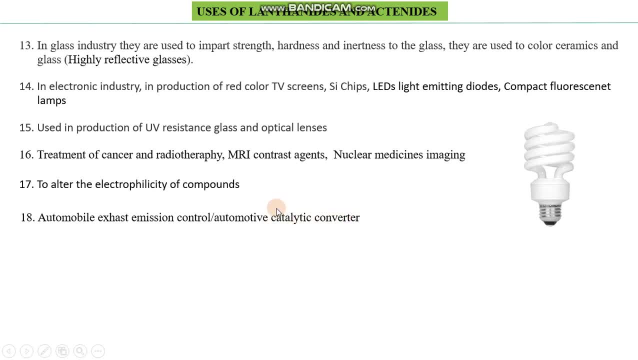 our environment. so this converter ensures complete oxidation of carbon in order to give carbon dioxide and to eliminate or to minimize the production of carbon monoxide which is the result of incomplete combustion during the automobile exhaust system. so they are used as catalyst in automobile, the catalytic converters. they can also be used in oil.